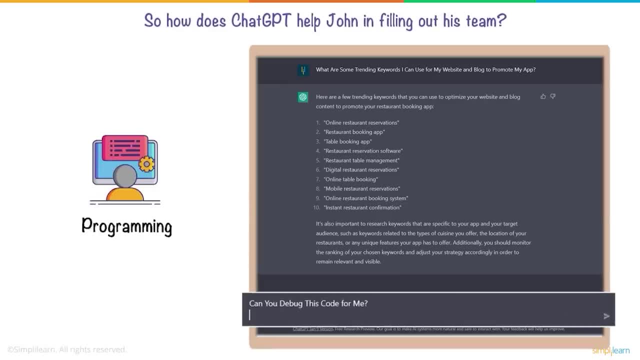 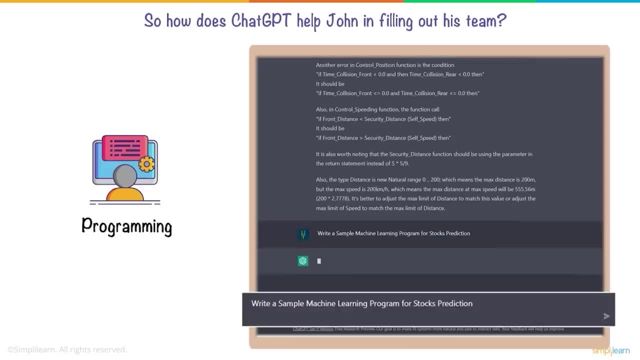 Speaking of websites, since John can do a lot of the heavy lifting in programming, ChatGPT can help proofread the code and help out when looking for bugs to fix. Apart from basic bug fixing, it can also provide sample code structures for different programming. 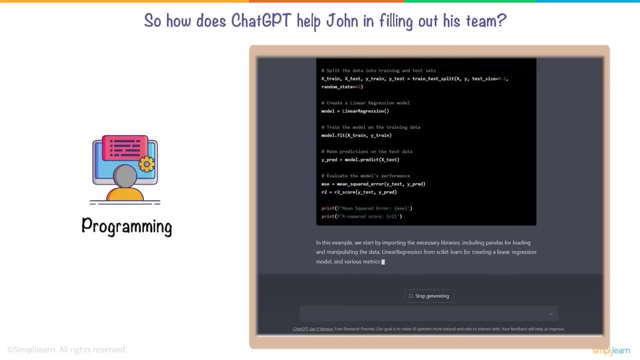 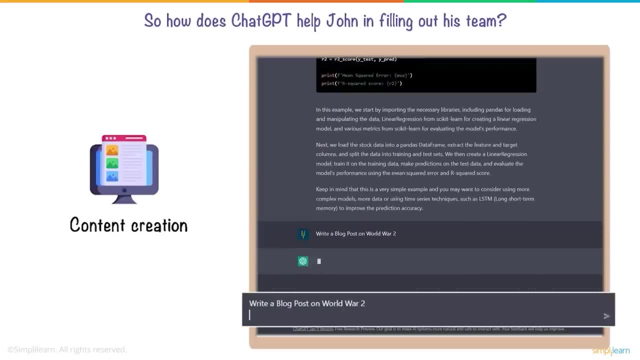 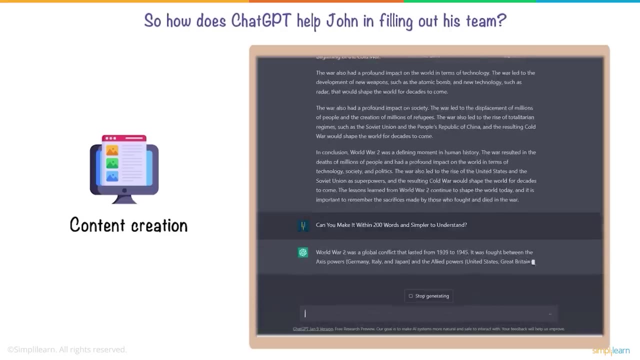 languages, allowing John to focus more on improving core functionality and workflow rather than fixing basic code errors. Websites and blogs' content is very helpful in gathering potential customer leads. The revolutionary bot can provide full-length blog posts with near-perfect fast accuracy- in seconds, allowing further customization, like 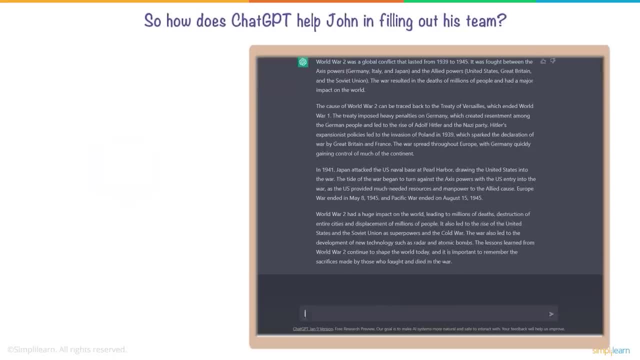 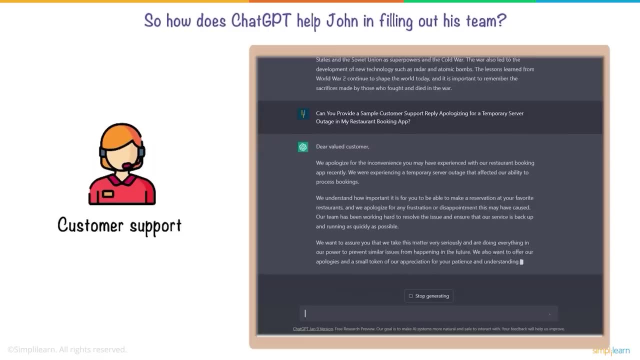 choosing the length of the subject matter to the complexity of language. For John's customer support, the bot can draft complete customer service emails based on the situation, saving time and resources. The tone of the message can be changed to reflect the nature of the message. 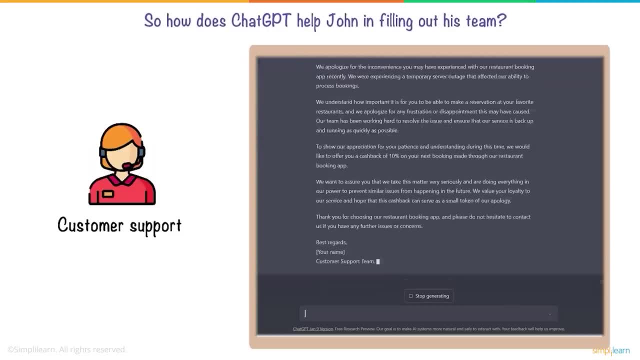 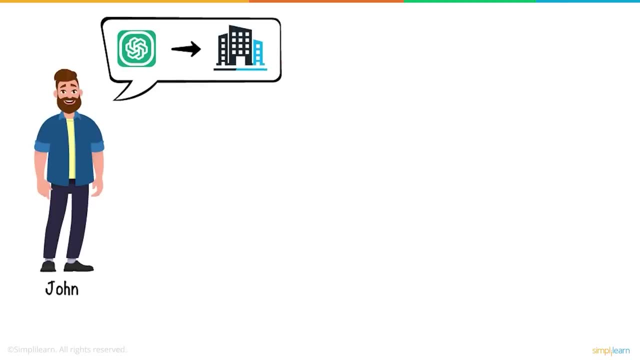 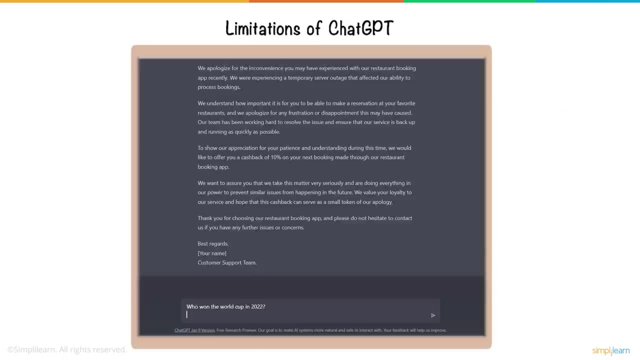 creating an efficient alternative for call center professionals. John was left speechless seeing this level of versatility from ChatGPT and wanted to implement it right away. However, Ryan made sure John knew about some drawbacks of the chat bot before getting started, Since the bot is trained mostly on data up to 2021,. 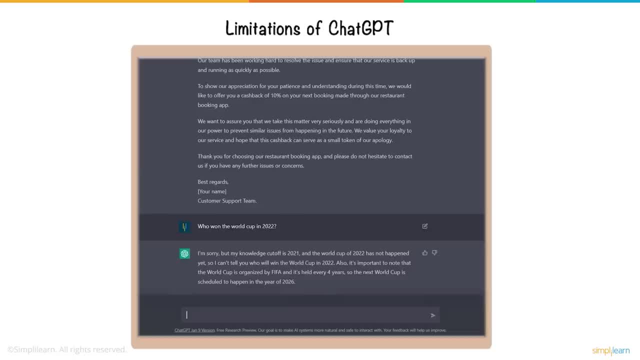 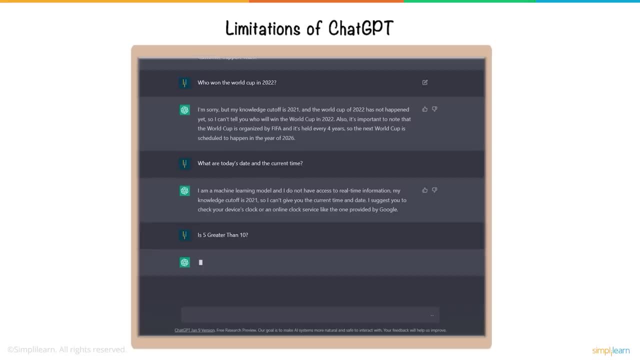 many of the newer events may still need to be discovered by ChatGPT. Even basic stuff like asking about the current date and time is beyond its scope, much like the limited understanding of context. despite providing near-lifelike solutions to certain problems, Even the accuracy of many responses can be questioned, since the 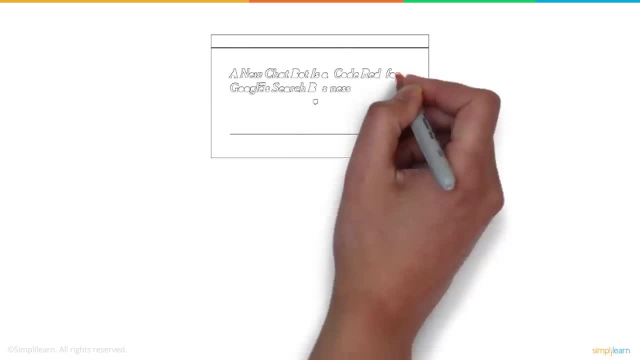 AI model is still learning and being developed. There is a section of the public that believes the revolutionary tool of chatgpt is the best way to get the most out of chatgpt. but it's not the only way to get the most out of chatgpt. 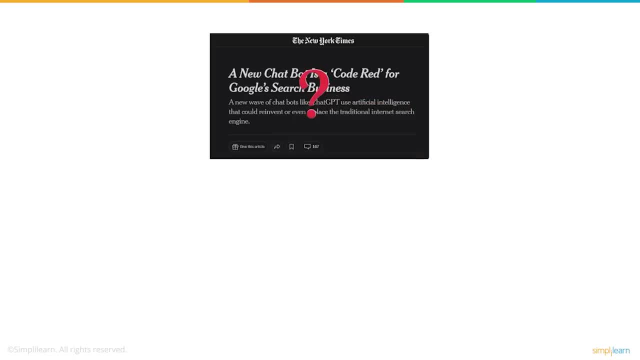 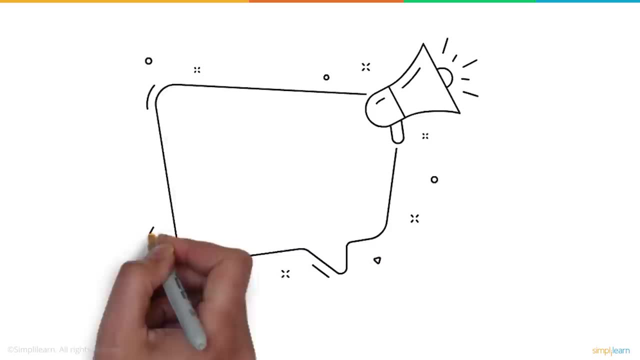 There are a number of other ways to get the most out of chatgpt, but that day seems far-fetched so far because of the variety of issues people keep running into when using chatgpt. So here's a question for you. Which of the following tasks cannot be carried out by chatgpt? 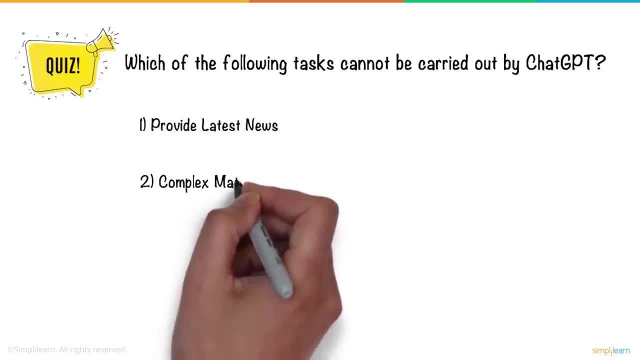 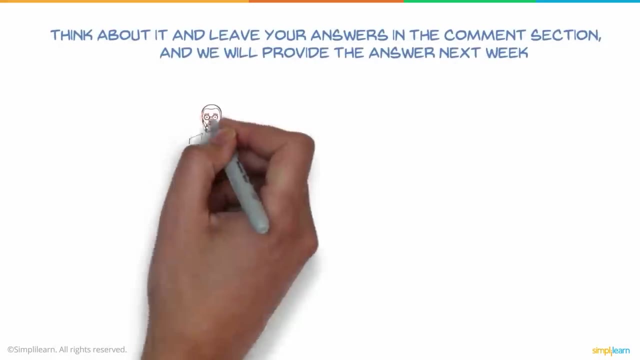 1. Provide latest news. 2. Complex mathematical calculations. 3. Food recipes. 4. None of the above. Think about it and leave your answers in the comment section And we will provide the answer next week. Give the correct answer along with your reasoning.